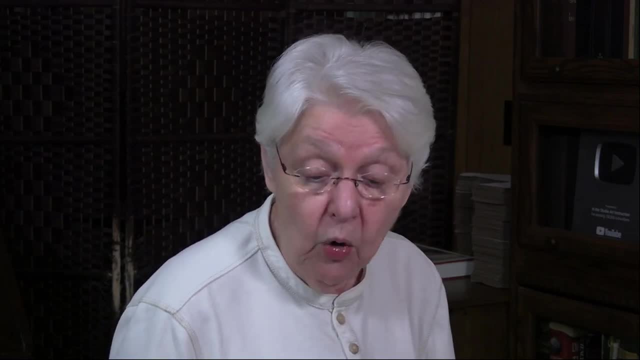 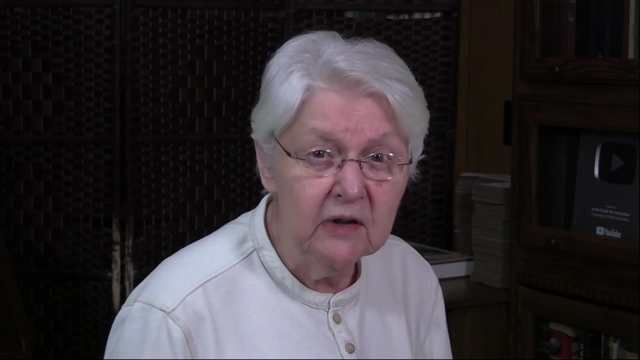 Well, this person says: I'm wondering how to begin an oil painting in regard to values. I learned to paint in the dark values first, but my paintings lean too dark. Can I start with the lightest values? Would that help? Well, that would probably do more harm than good. 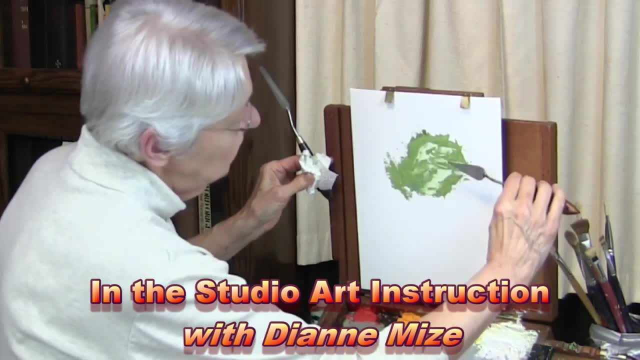 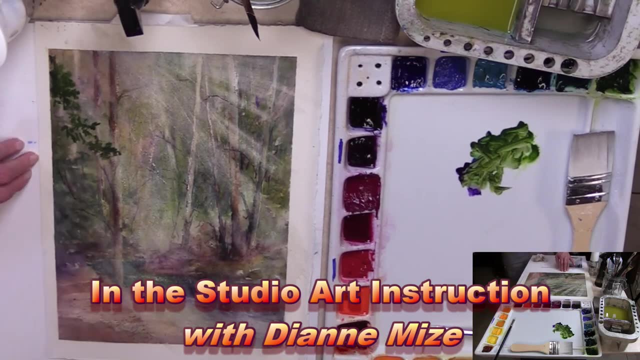 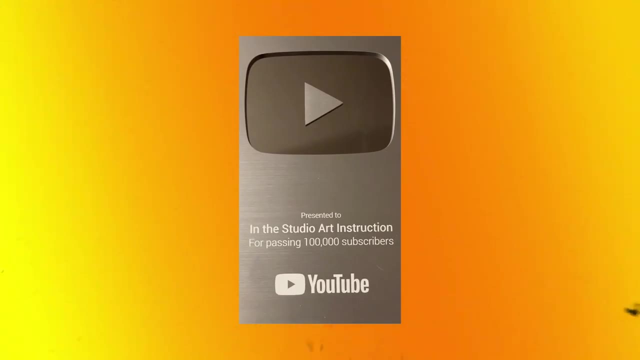 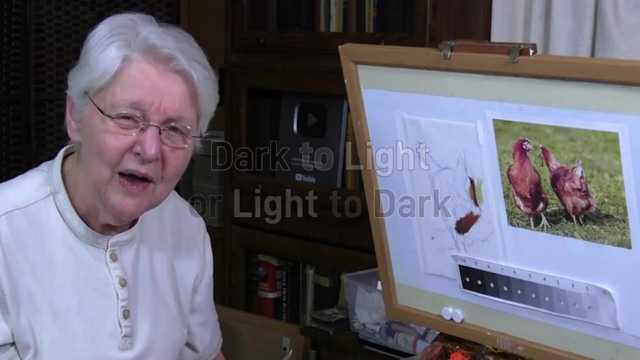 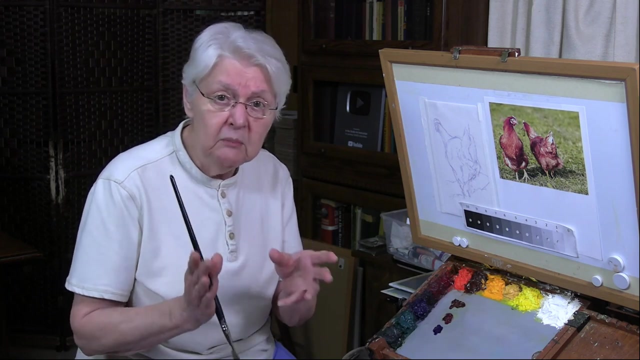 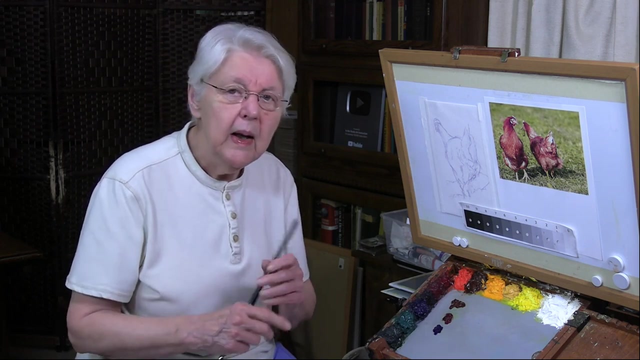 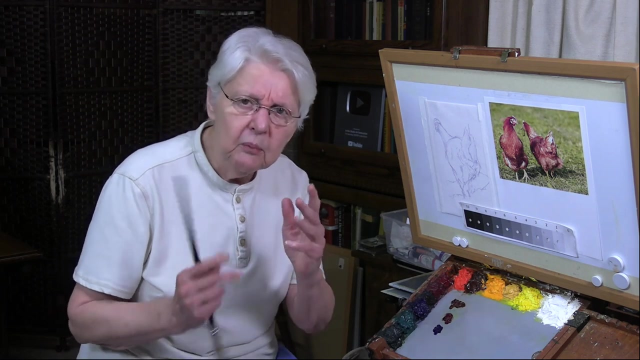 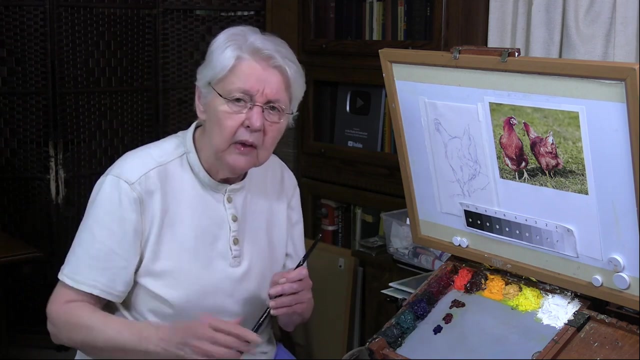 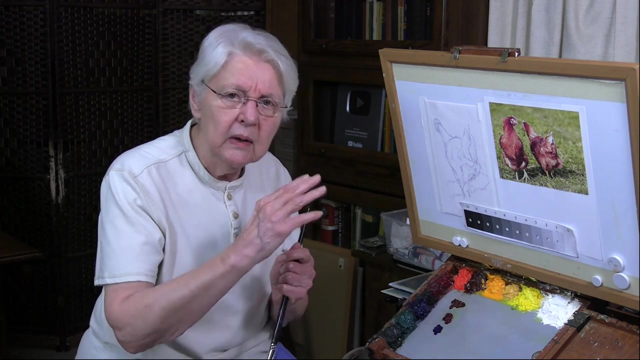 Well, there are two reasons, really, why your painting might be going too dark. One could be a very simple one. Now, whether you're painting in oil or acrylic or watercolor or pastel, it doesn't matter what- If your studio lighting is too bright, your tendency is to make your paintings too dark. The same is true if you're painting in plain air. If you paint in plain air, in the sun, without any kind of shield, anything to shield the light, your paintings are going to end up too dark because the light is going to make you think that you see it lighter. 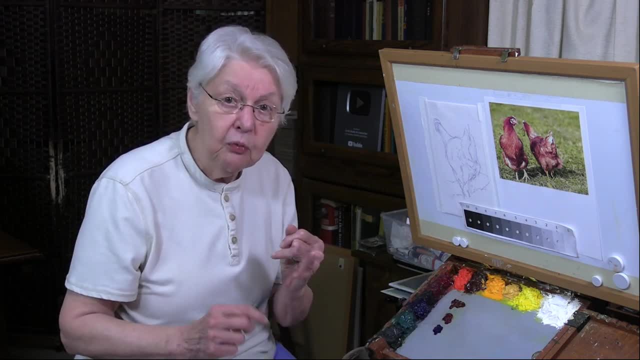 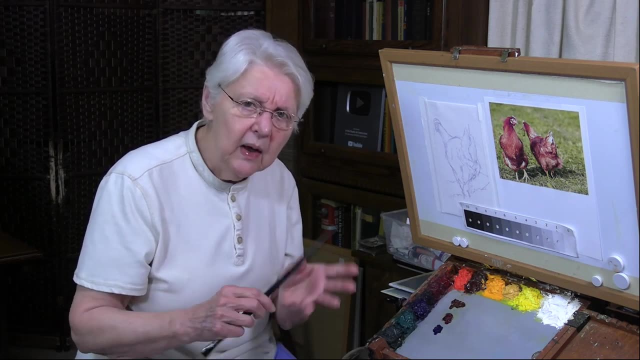 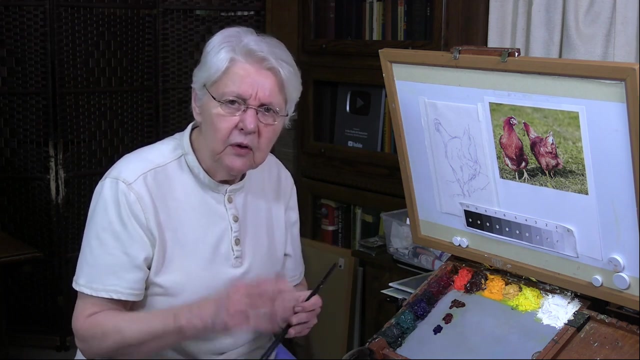 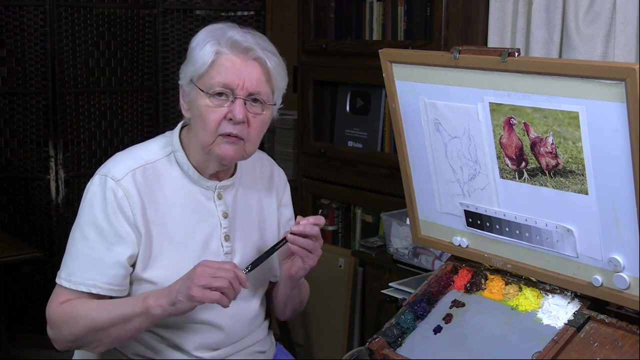 So we have quick tip 306 about lighting for those who are working in studio lighting. that guides you about how to control the amount of light that you actually paint under. So that is really, really important. And those of you who are plain air painters always paint under some sort of a light shield, a white umbrella or some way to shield the light. 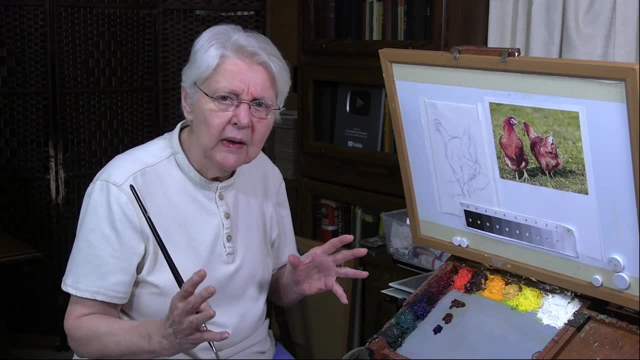 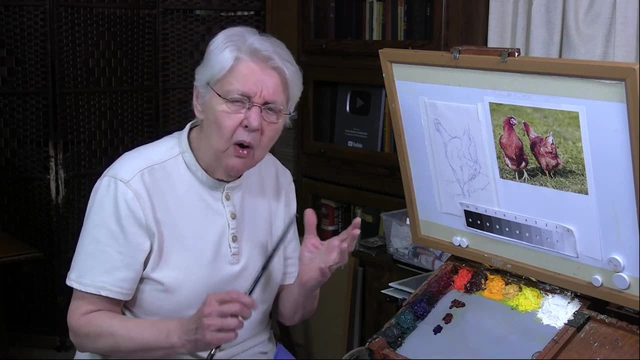 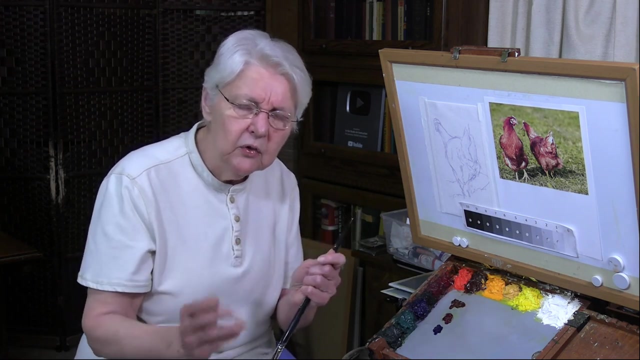 so that you don't have that bright, bright light that will mislead you about your values. the other one is unique to oil. now, with watercolor, the approach, technical approach, we use with watercolor generally is light to dark painting, light to dark. in acrylic the problem doesn't exist because it's. 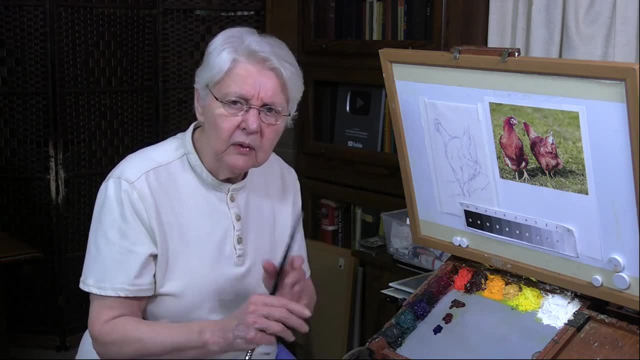 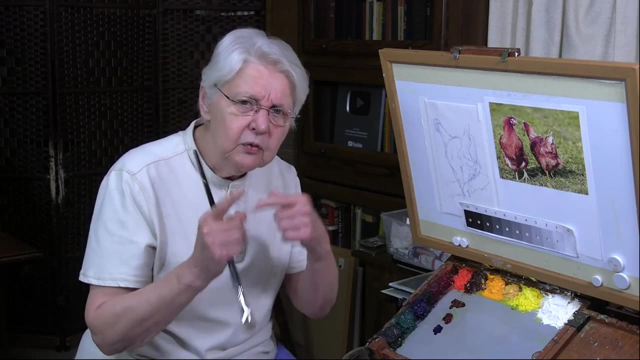 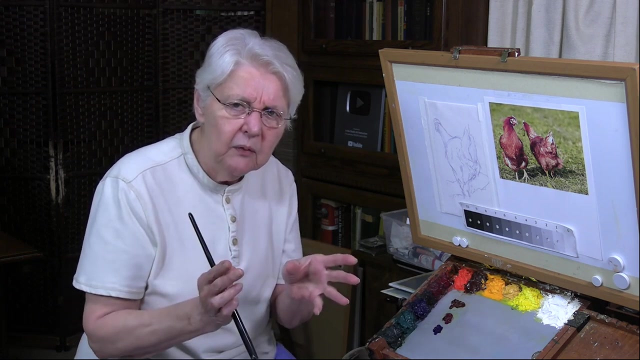 a technical problem with acrylic. if you start out with your lights, then there that paint is probably going to dry before you really start putting in darks. but structurally, even that you will come nearer to getting a well-balanced painting if you begin with the darks. that's not the answer. 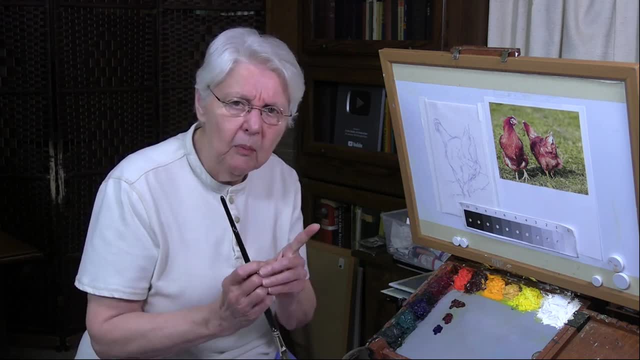 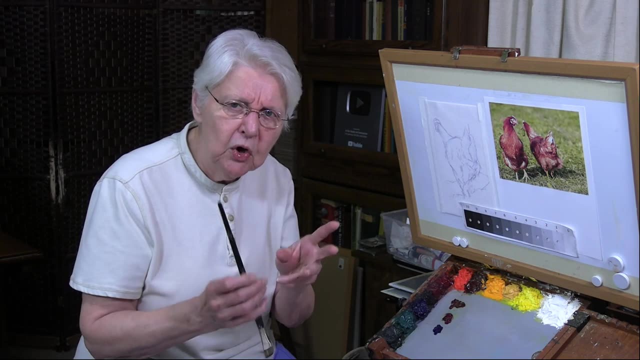 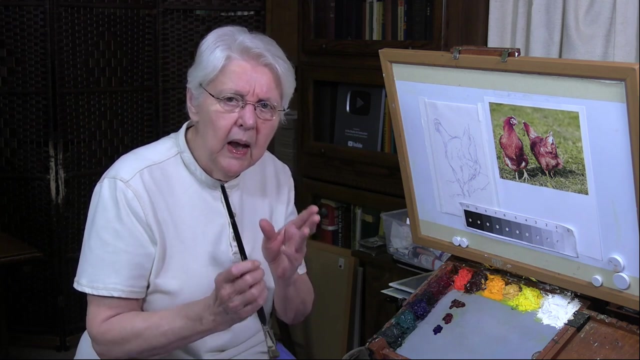 to the question. the answer. the question is specific to oil paint. what happens with oil paint now? it's very important. one thing is that you learn to see the values that you're mixing, because if you see the values your mixing and in in relationship to where they belong on the painting, then you will come nearer. 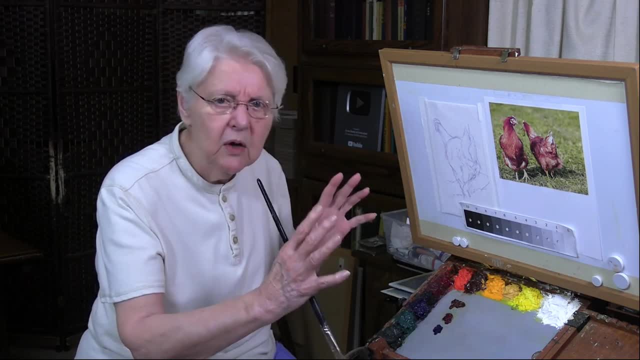 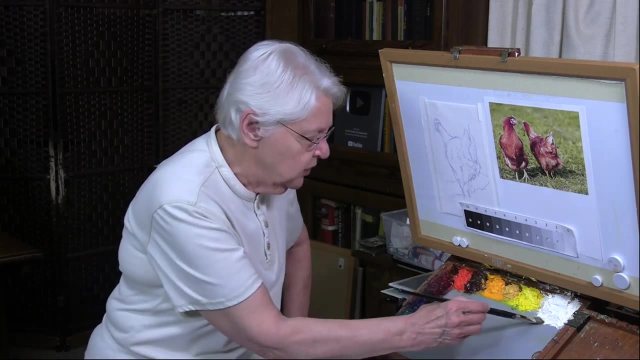 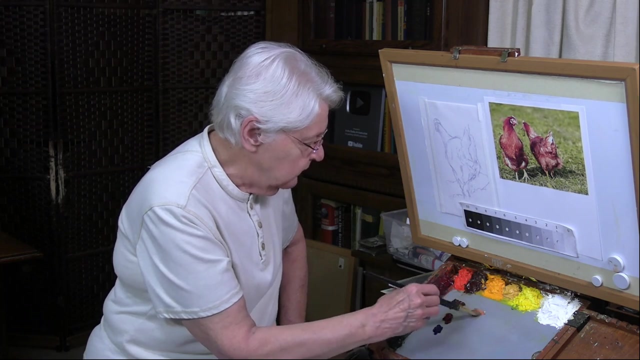 to being able to control that business or make you'll be able to make your lights light enough. so I'm going to take it from two points of view. one is this: if you make an area too light- and I'll just show you that right here- let's just I'll just randomly grab a little color and let's say: 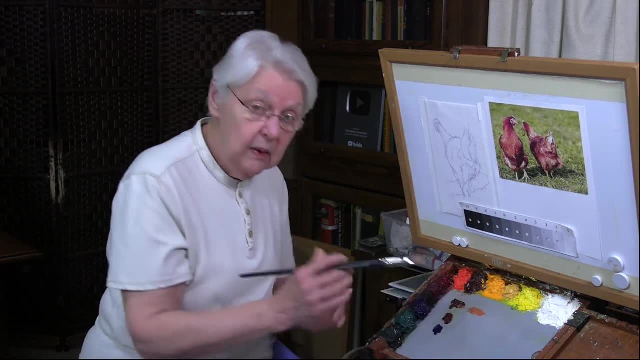 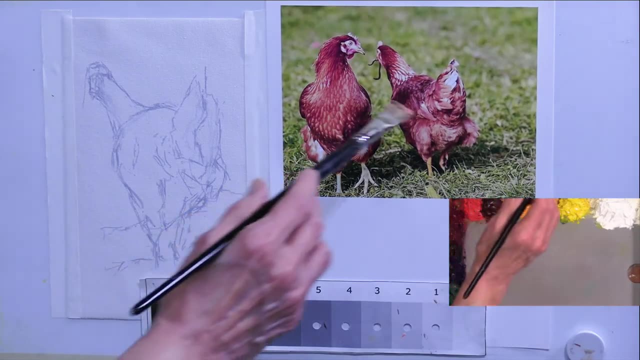 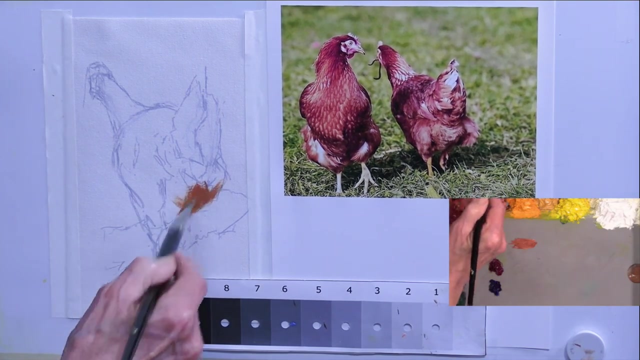 if you make an area, if you were to start light and work towards dark. here's the danger, here's the yeah, danger that you run into. say, if you had an area, say like a shadow area of that chicken right there, and if you made it this light like that. or if you make 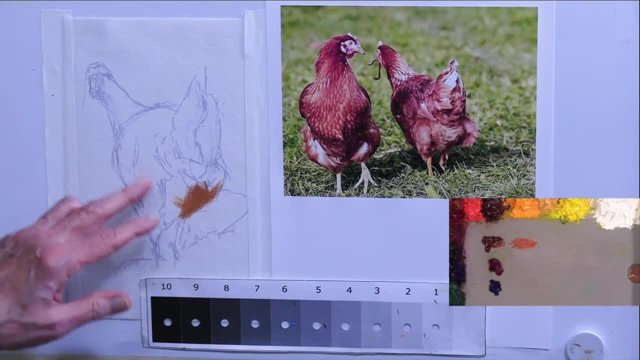 that value. you think, well, that looks down dark enough because you see around it. you have the white canvas and you think that's dark enough and then you discover it's got to be darker. if when you're trying to make that light, when you're trying to make that dark darker with oil and 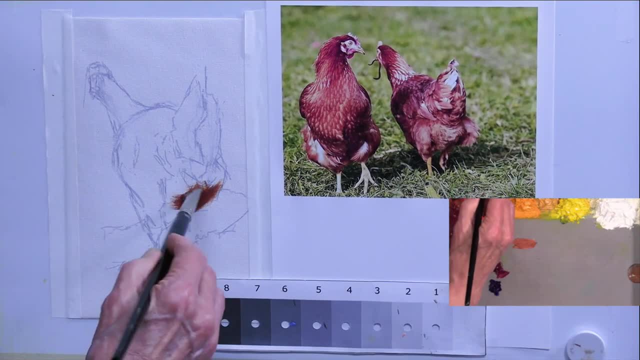 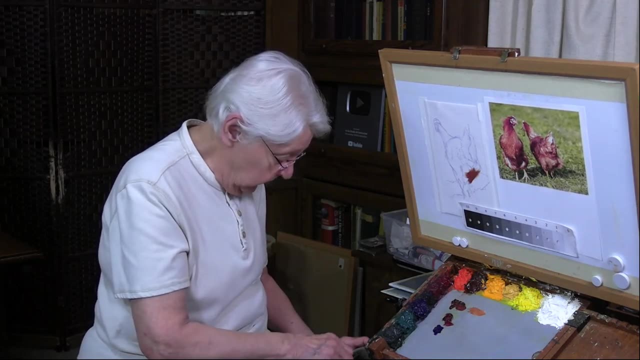 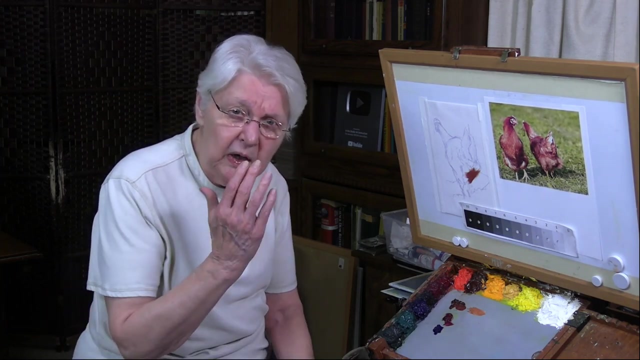 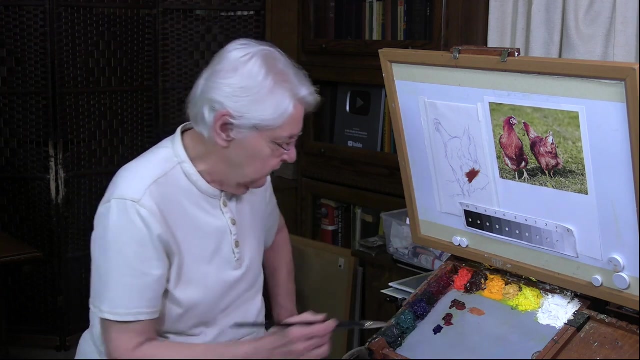 the darkly you put in there tends to want to get muddy. it's not as clear as the dark is if you have it darker, and I'll show you that. if you start out darker and make it lighter in oil, the dark is clear, it doesn't. it doesn't have that tendency to go so muddy, that is, unless you brush it to death. so 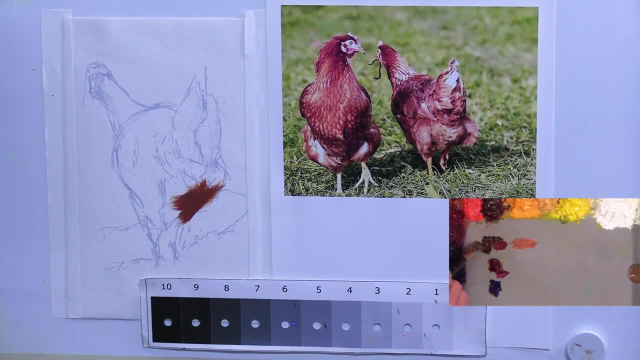 if I started out too dark in an area, let's say in areas such as: let's just put: I'll just do something like right here. so so if I started out too dark like that and I saw then that it was too dark and needed to be a little bit lighter, 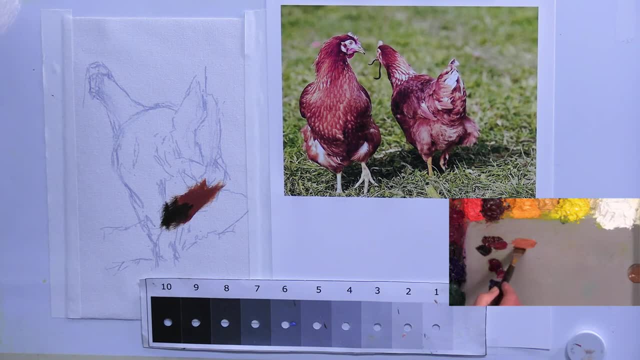 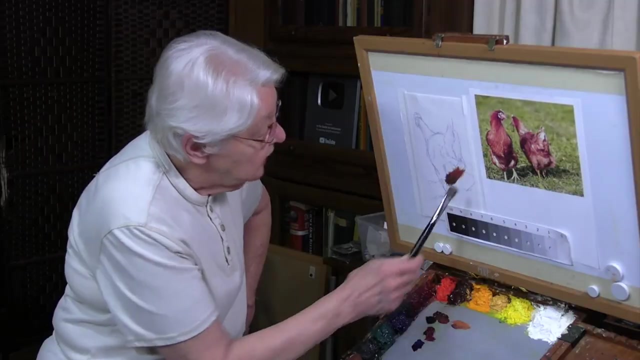 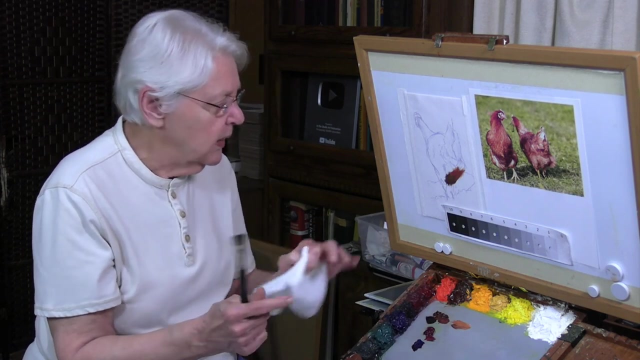 because of the nature of oil paint, I can make it lighter without it getting muddy. I can make it lighter and it still retains its its brilliance, and so let's see if I can get it about the same value as that. so you see that there's a technical reason there why oil works better if you work from Dr light. so 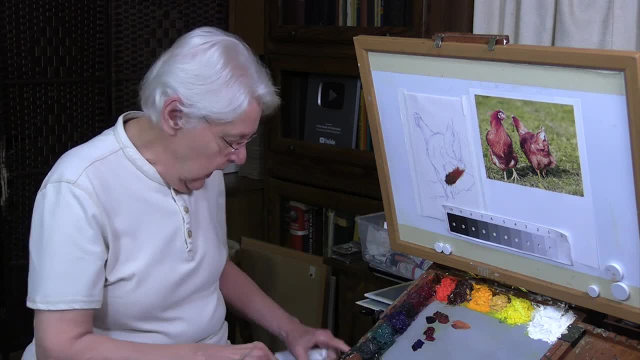 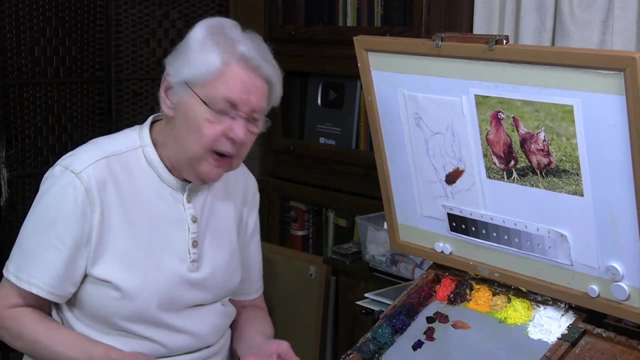 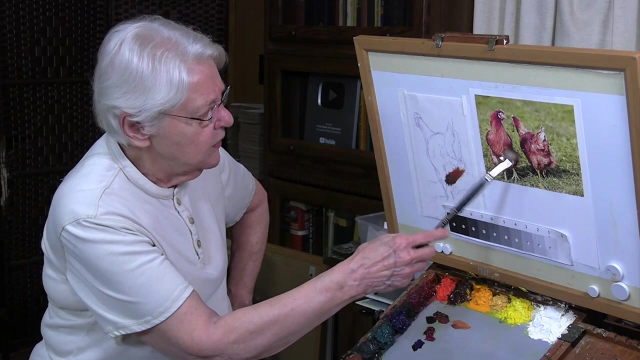 let's now let's get away from the technical reason and look at how do you really see the values that you're putting there. if you learn to see those values correctly and learn to mix them correctly, you're going to be okay. so if we look at the lighter now, I want to just use a portion of this. 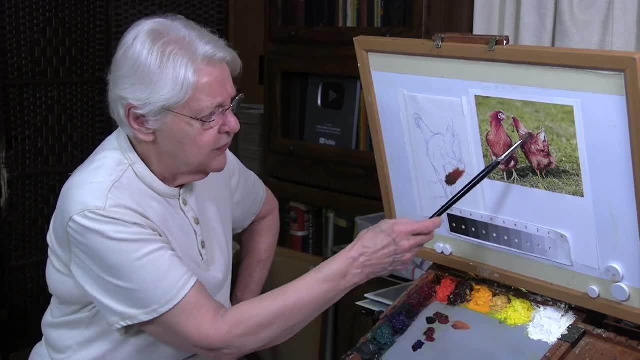 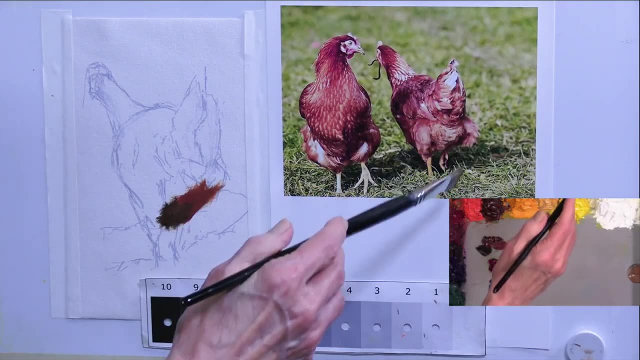 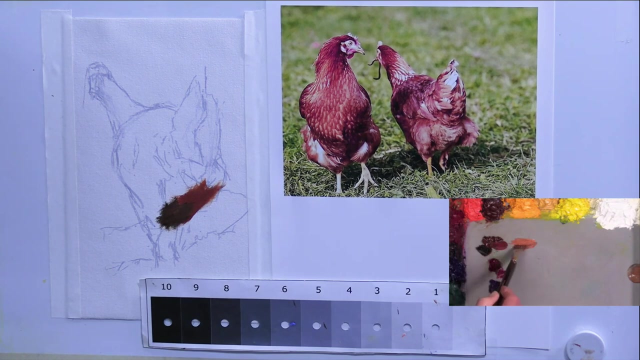 because it has all these values in it and it also has the lighter values around it, which is one thing I really want to address with you. all right, so suppose now, uh, you're, you're painting that chicken and and you've made the value, you've got the values on the the um, you're working dark. 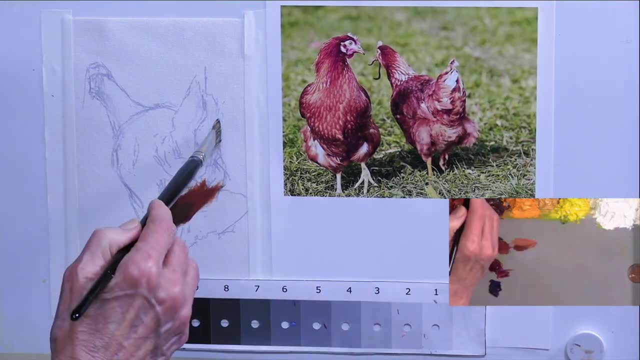 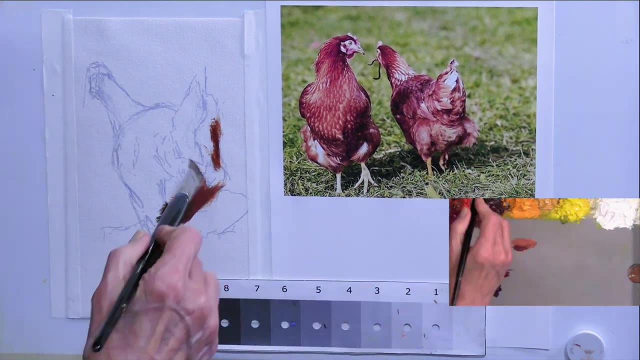 to light. let's say, you're working dark to light and so we have this really really dark value area right here, like that, and let's see you guys, there we go. so if it's not the darks that you're having trouble with, you've got that area like that and then you're 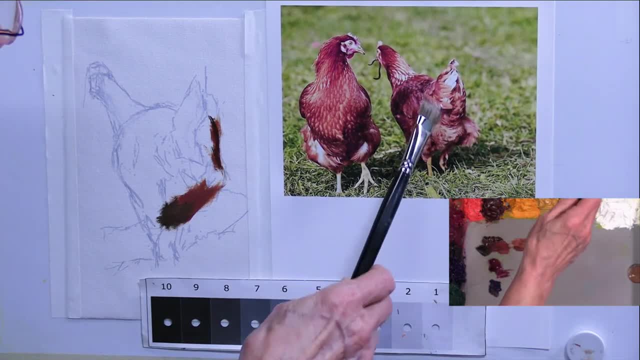 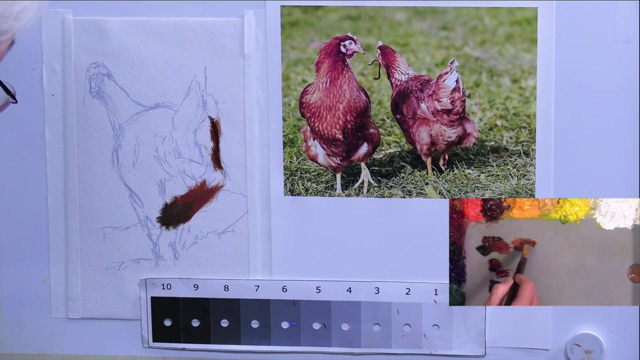 getting a little bit lighter. how can you be sure that this light here and this light here are light enough with what you can be sure is by comparing. so for one thing, you see the light right here if I mix that light, this lighter area right here. so let's say I'm trying to get that light and if I have a tendency to get too dark, 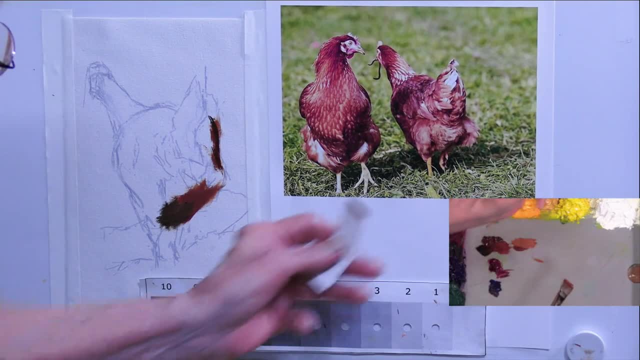 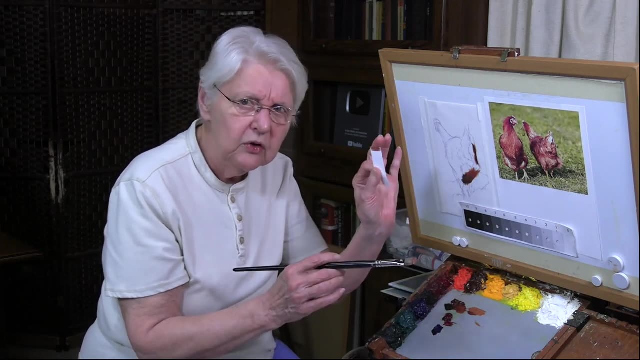 one way I can correct that. I say, okay, that looks light enough against my pet, this will not light enough. I hold it here and I see it's too dark. so one one really really good way you could do that is use little test strips like this: three by five cards you buy in dollar store, maybe about 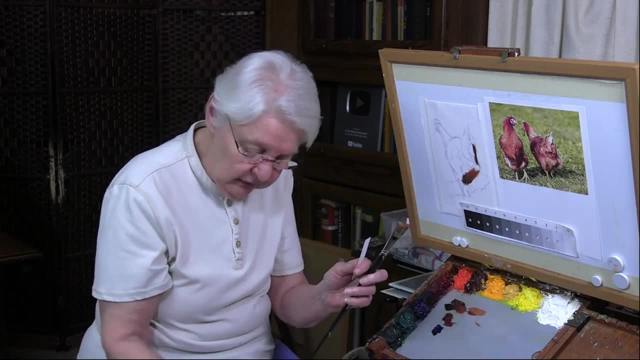 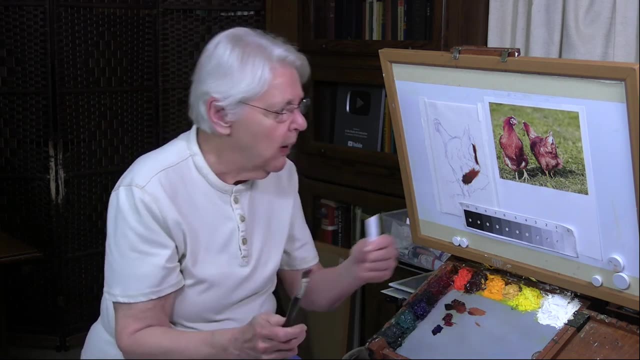 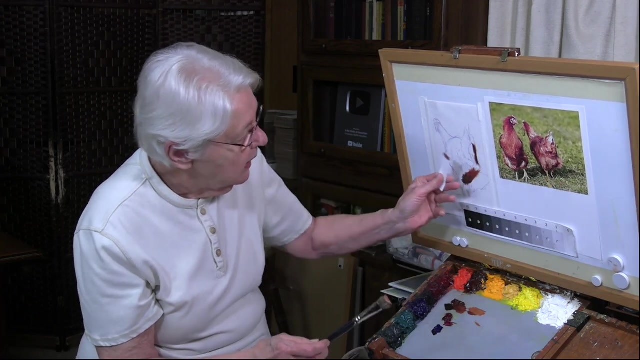 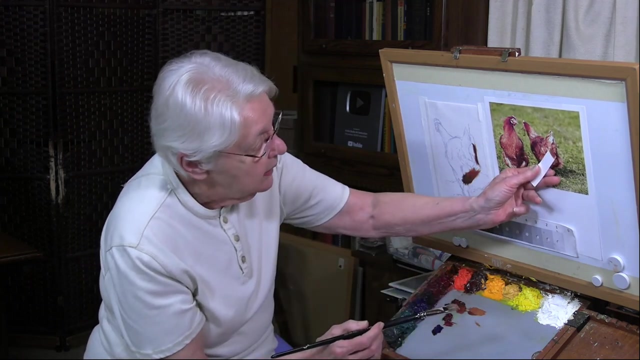 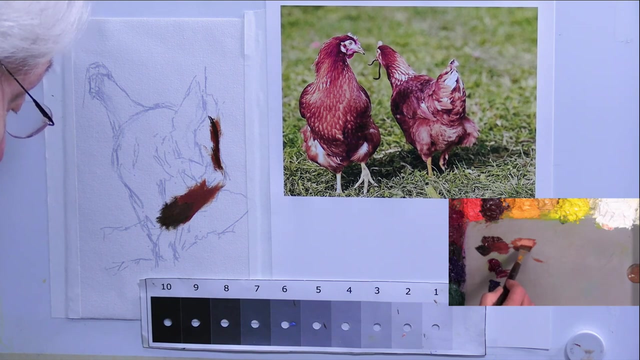 a buck a pack. just cut them into little strips and carry them with you wherever you go, and then you can test out. I'm gonna put that one with some press before I put that back in. come on, come on, I can't do this better, can you see? it's really too dark. now that is quite heat sensitive. when you're mixing color and you're trying to control, you're trying to solve that problem rather than gas. always test it out before you put the color down. you see that's way too dark. it may look light enough when I first mix it, but it's way too dark. 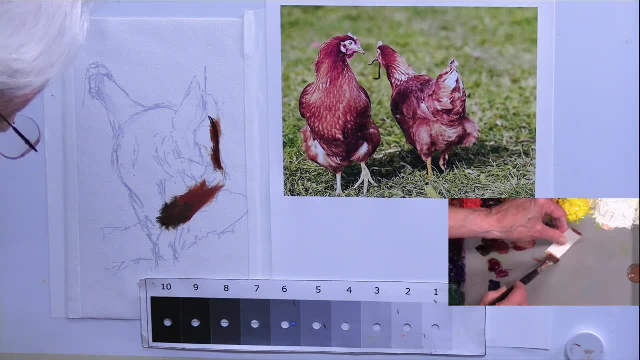 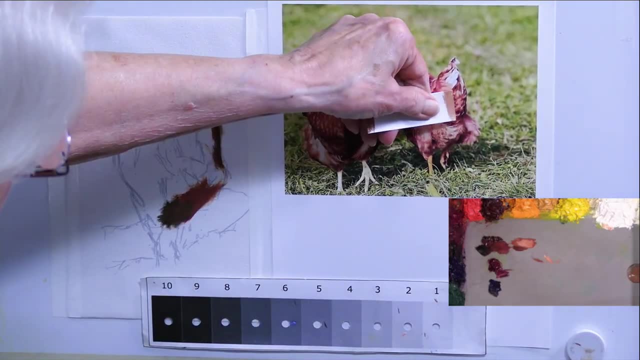 so then if I do it that way, you see, I see it's too dark, then I can lighten it some more and test that. now test: always use a clean area when you're using test strips. Now let's check out that value. You see, that's closer, That's closer to the light value I'm seeing there. And so then if I put that value, 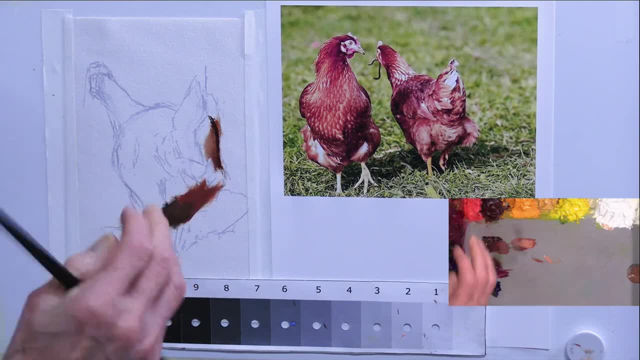 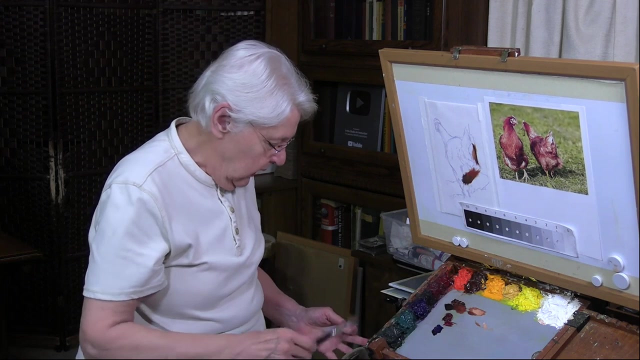 here. you see, then that looks that enables that light to look lighter, because I compared it and I'm comparing the dark to the light and I'm able to see that. What about this? It could be the ground you might perceive to be light, but you're really making it too dark. 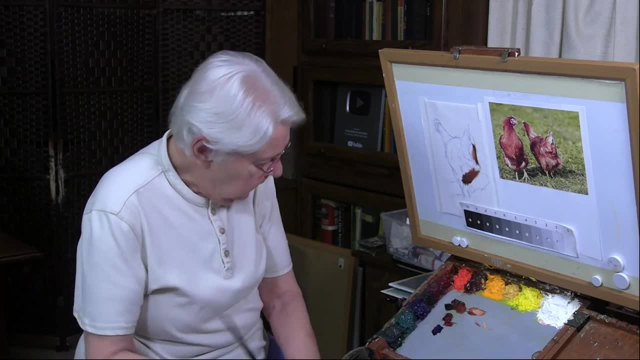 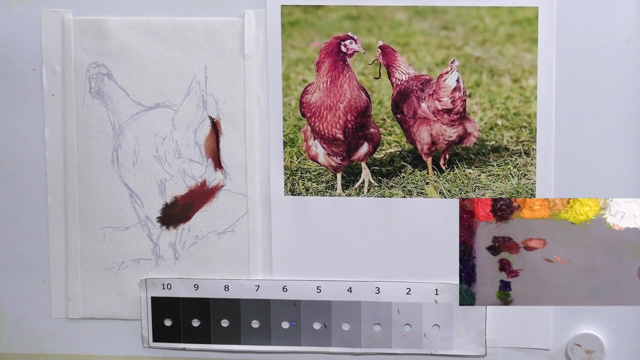 You'll use the same method, but let's just show you here, So I will. let's just get ourselves a green there Now. if I'm looking at that, I can detect- and you can too- that this is lighter than the area right here. So I see it's lighter. How much lighter is it? One way I could. 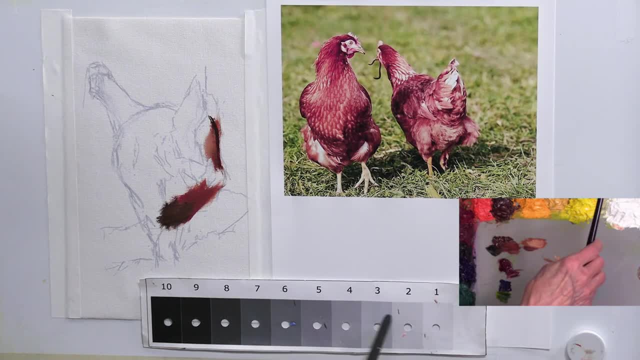 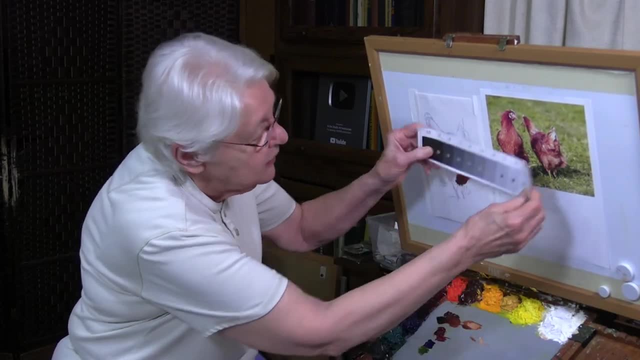 do that is if I use the value scale and check it against the value scale. So if I move the value scale now, see, I've got little holes punched in my value scale. so I could hold it. you know, I could hold it like this and close one eye and do that comparison if I'm working plain air. 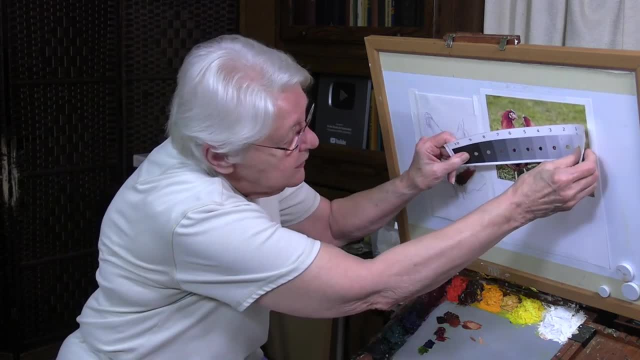 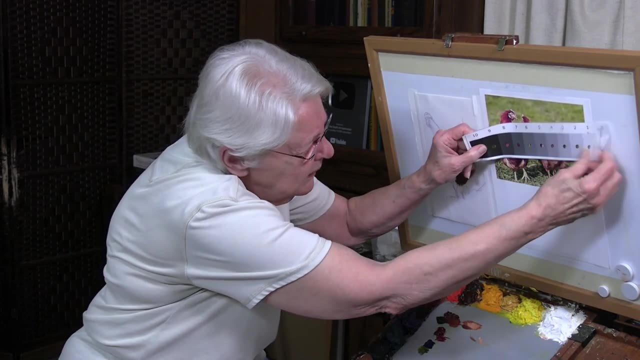 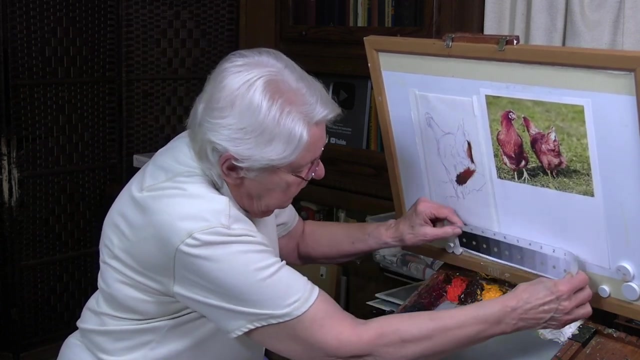 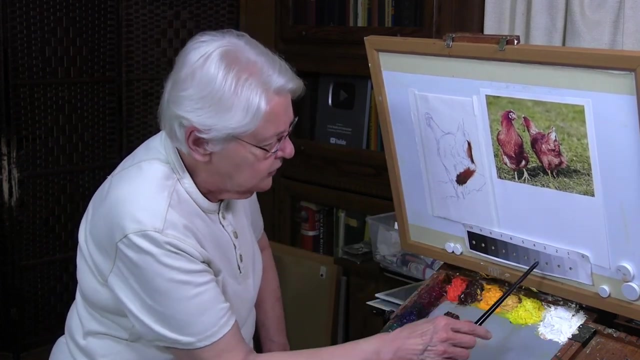 which does help. But see, if I do this and I say, look, well, it's a little bit darker than this value, well, it's about the same value as this value. So this is a value I'm looking for right here, and so when I'm mixing, then I can mix, for I can mix towards that value. Let's see, let's do that. 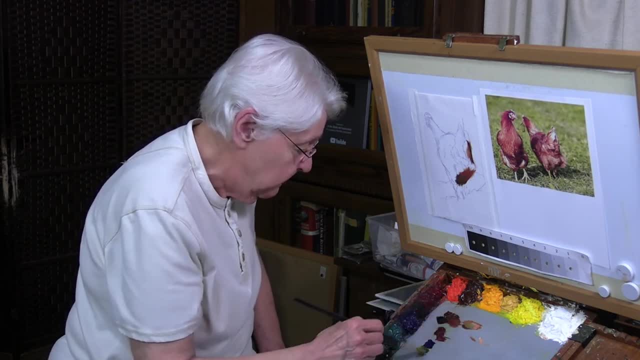 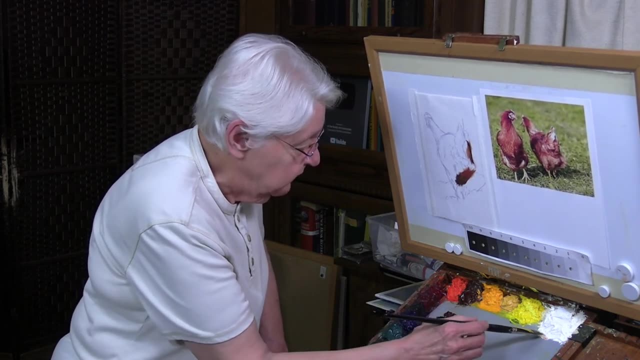 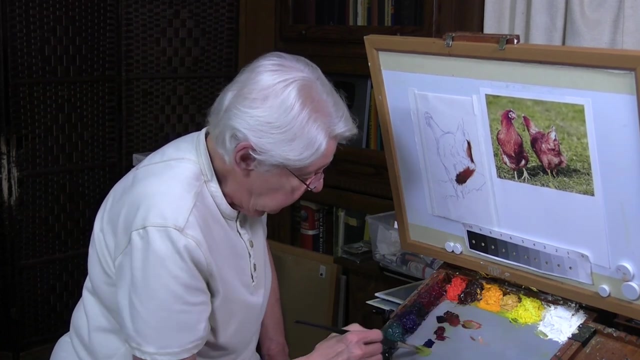 You see, I'm showing you two methods for going about this now. and so let's just pull some more yellow into that and you see, that obviously feels a little bit dark, But now it's beginning to feel lighter, because it's lighter on my palette and I might think I'm 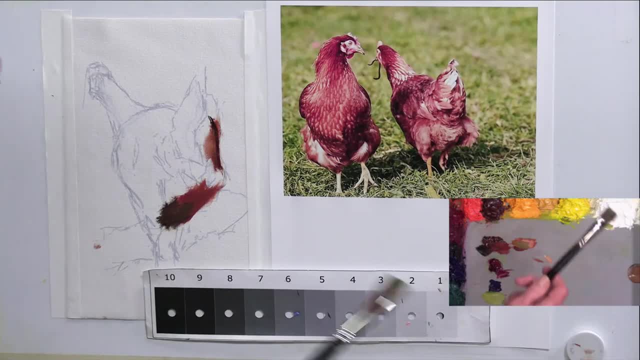 light enough, but am I All right? so if I read that value, it's this value. and then another way I can do that is to double check. I can hold my brush, I can mix a color, mix a value of a color. 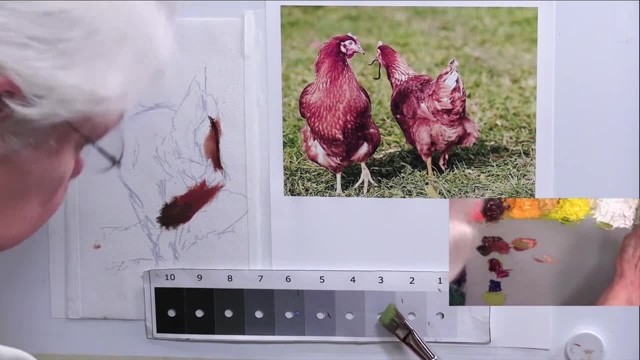 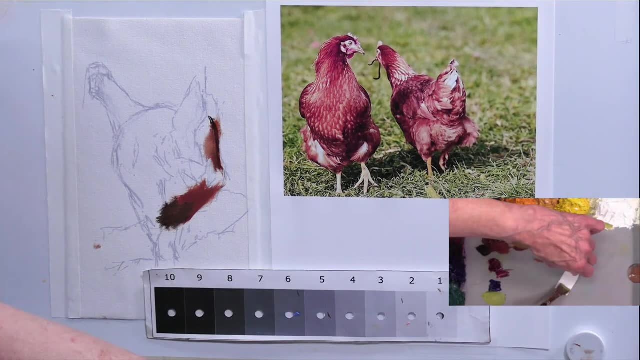 and I can hold my brush against the color, the value scale, and I can squint. And does it look too dark? Then I can squint. I can also hold it this way, or, once again, I can do this now, and it: is it too dark? is it too light? is it just right? you see, it's too dark. so. 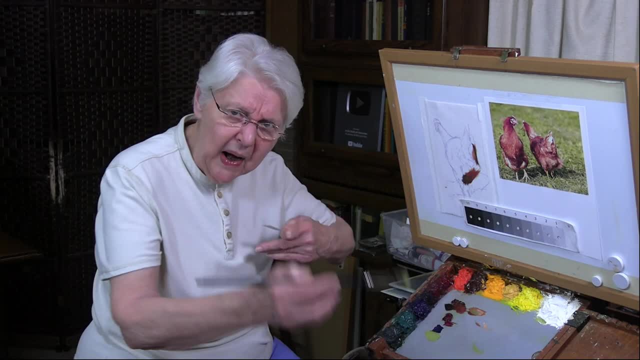 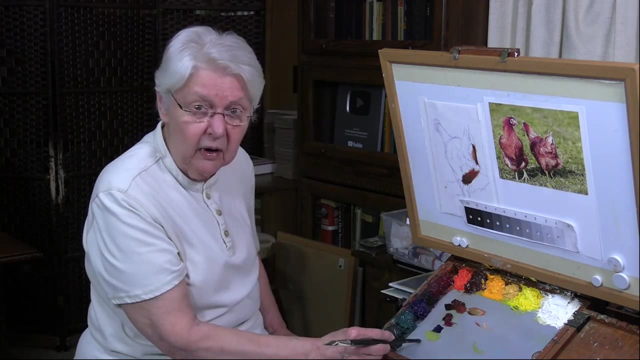 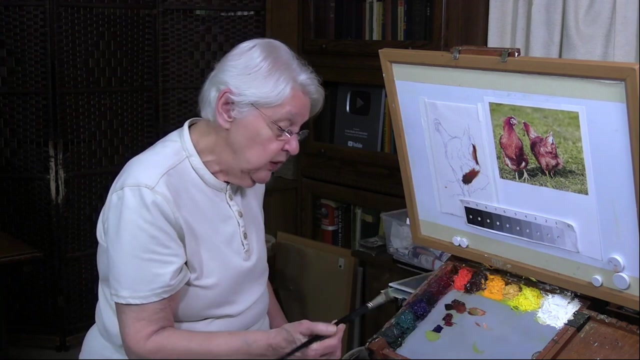 see, that will tell you if you, if you use a comparison method like that, where you you think it's light enough, it looks light enough on the color wheel, but then when you actually make the comparison, ah, it's too dark. so then if then you force yourself whether you think it should be, 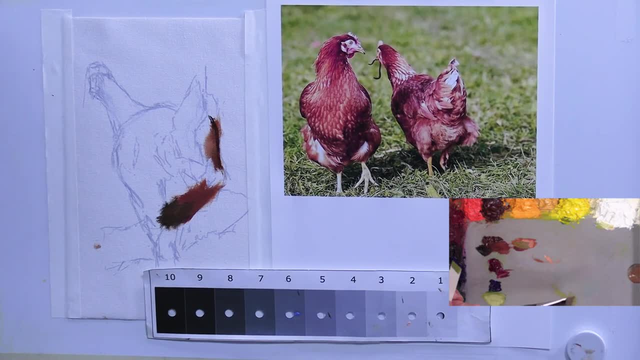 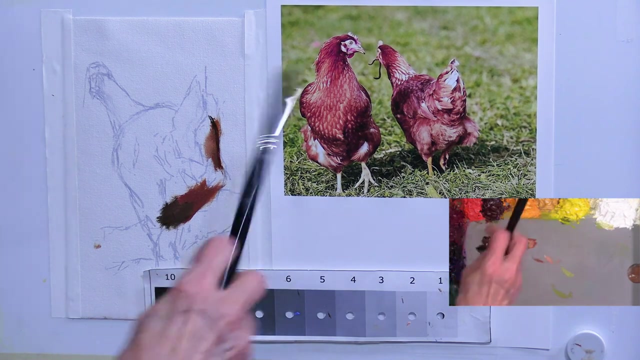 that light or not, you force yourself and make it lighter. and let's use a fresh area on the, on the test strip here and now. let's compare that. that that's close, that's pretty much in that light value range. and so then if we place that here, it's going to, it's going to be light enough, you see. 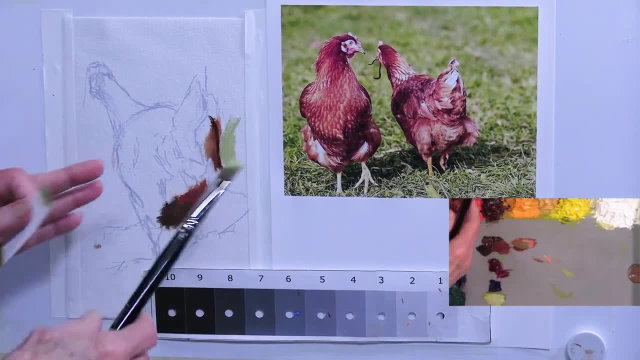 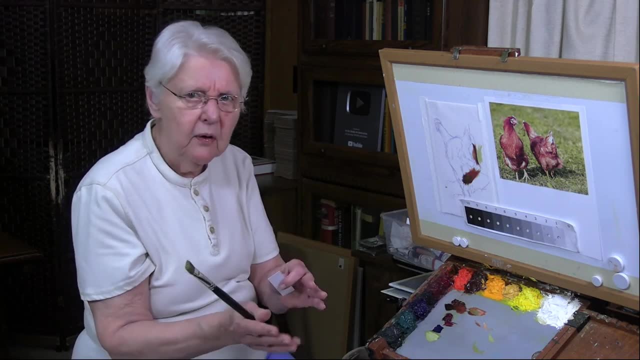 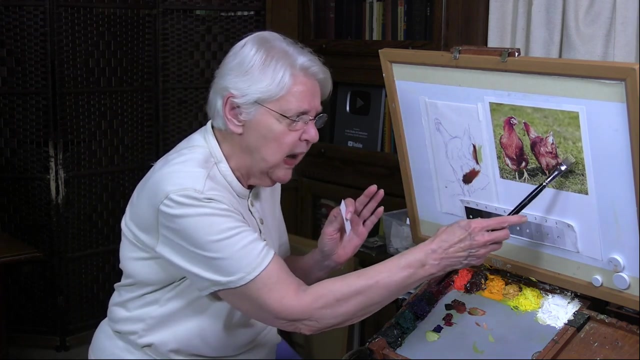 what we've done there. so we've got that value comparison. of course, when you're painting on a white canvas, if it's not toned, if you put your darks in first, you will get that comparison always, because you'll have your darks in and you can compare the lights here with the darks you're seeing here on the other. 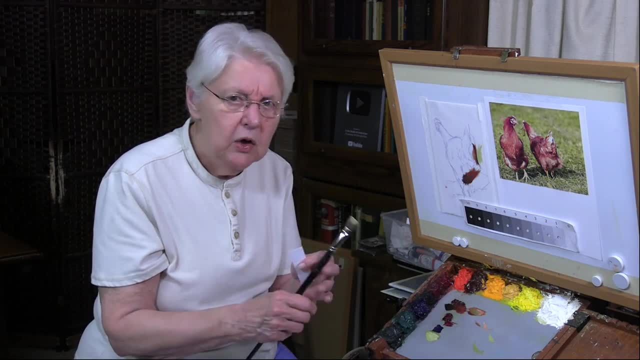 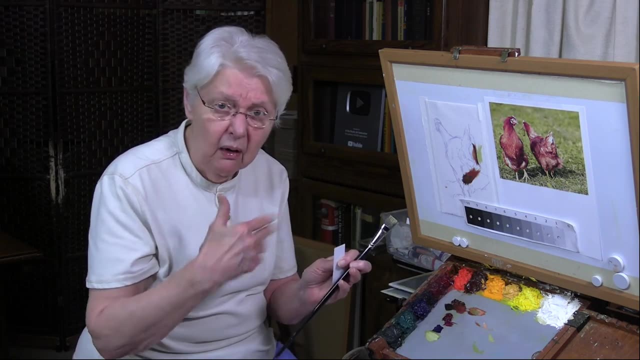 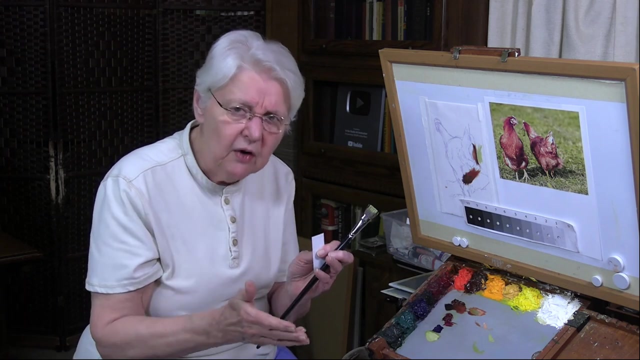 hand, if you start with your lights first, you have no way of comparing the lights except against the canvas and the canvases, unless you've toned it dark, and that's not always a good idea. but you have no comparison if you have your darks in there first, you do have that comparison, and so that will enable 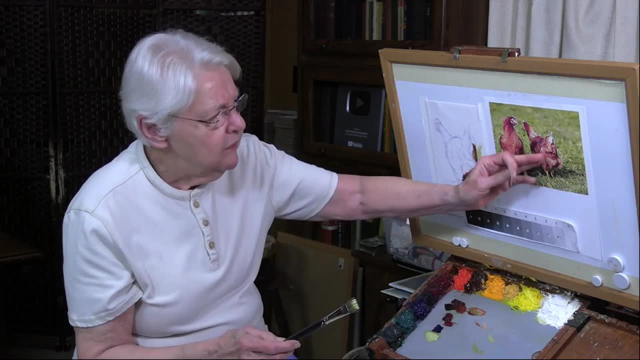 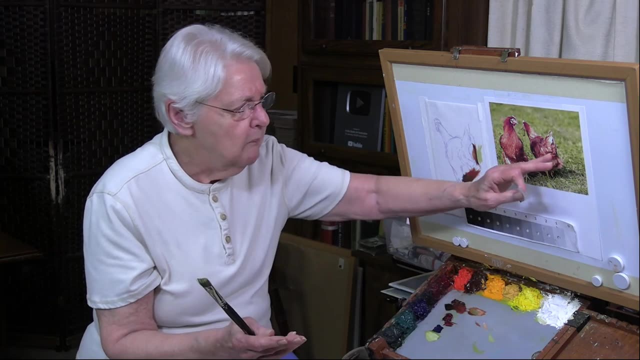 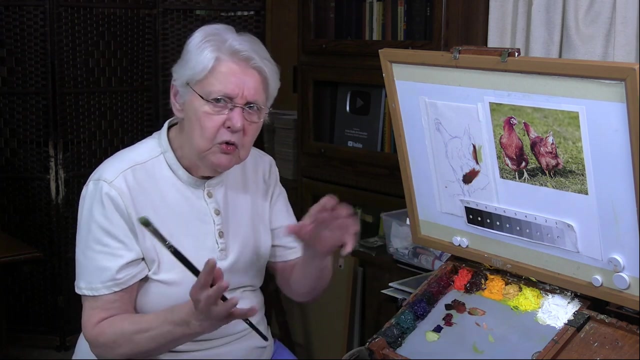 you to get those lights lighter. so i think maybe, if you will just slow down, do some practice sessions where you actually practice. uh, making this comparison, use these little test strips. they don't cost that much and they really are a help where you guide yourself just by asking the 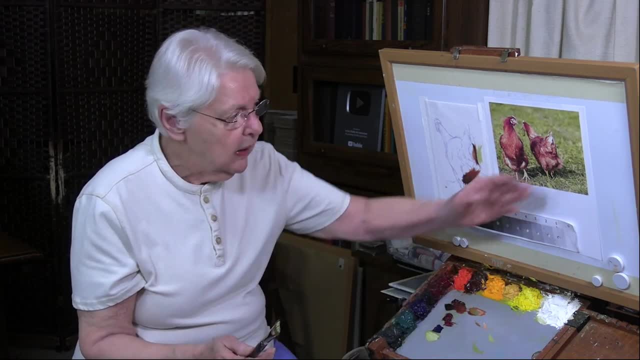 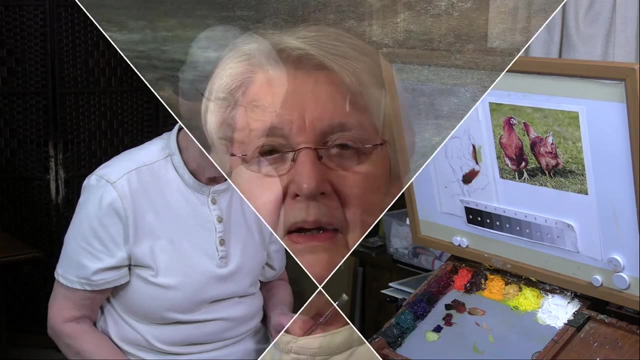 question: uh, when you mix the paint and compare the colors, and you can get a better idea of what's going on with the paint and compare it here, does it need to be darker, it doesn't need to be lighter. give that a try and see if that doesn't work for you. be sure, and view all of our quick tips.